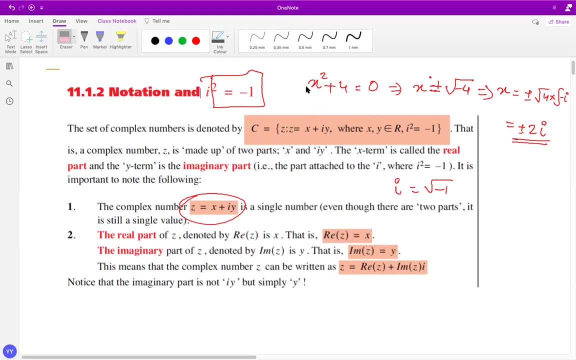 two i. So you get the possible solution, that's your non-real solution for the complex number. Now what we are going to do is we're going to first understand how do we do the arithmetic operations on complex number systems. We are going to take this general expression and then 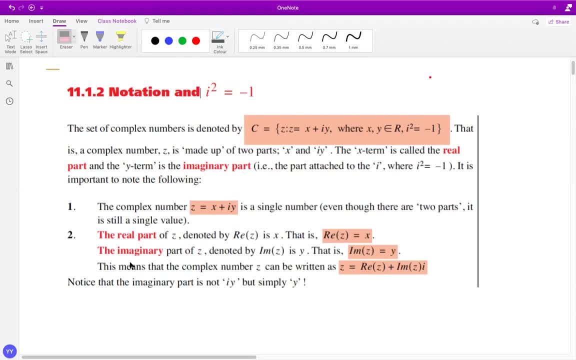 on complex number. So let's just begin up with first understanding what a complex number is. So a complex number is generally of the form X plus IY. So let's say, when I say something like okay, two plus three I, this is a complex number. 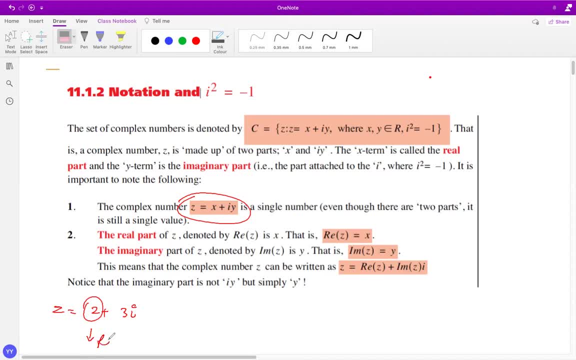 So two is referred as the real part. here It's called real part And three is called as imaginary part. So when I say that, okay, R E Z, real times, real part of Z is basically straight away two And I am part of Z is basically three. 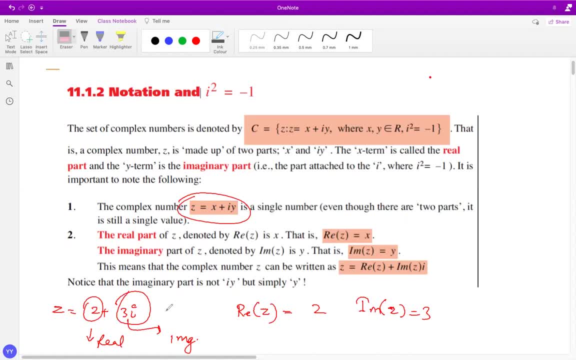 So lots of times people write down: I am part as three I so that's not correct. So imaginary part is actually three. So real part is two and imaginary part is three. So when I look at this diagrammatic presentation here, we have real axis X instead of X and Y. 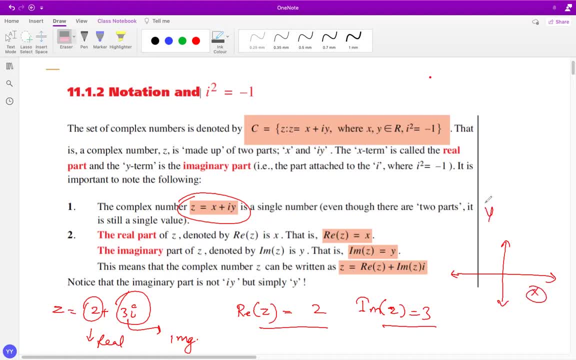 we got real and imaginary axis, So this is like Cartesian X and Y, So X is basically replaced by imaginary axis and this is called as real. Sorry, this is real axis and this is imaginary axis. So when you have real and imaginary axis, 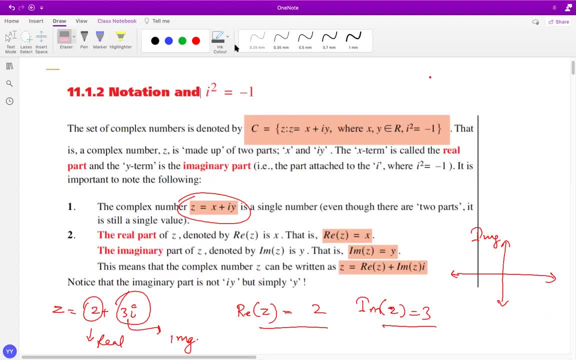 like for example here: let's say now, if I have to present this complex number, it's gonna be, let's say, two units like from here, like how we do for vectors, and three units here. So the complex number is actually located somewhere here. 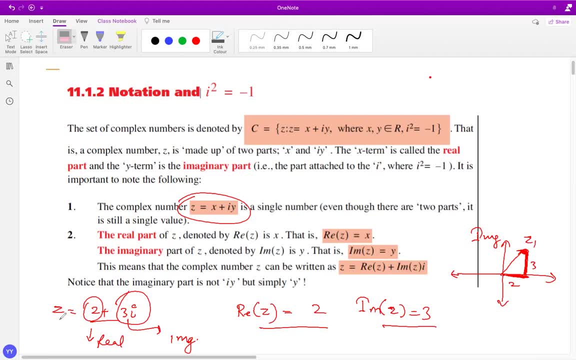 So this is actually the position on Z one. I mean, if my complex number is Z one, So this is referred as Argon diagram. So this is called an Argon diagram. So when you take on X axis your real part and on Y axis imaginary part, 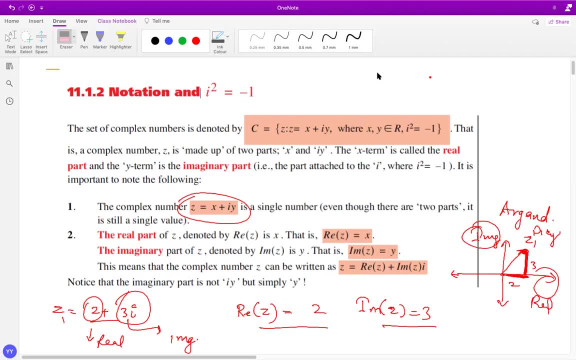 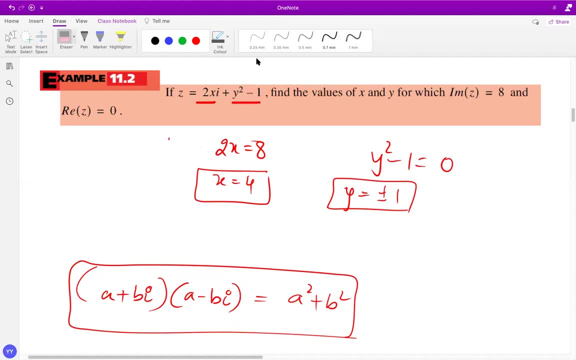 Now let's take out some basic properties of the complex numbers. So now here is a simple question on the property of complex number that it's. the question is that Z equals to two, X, I plus Y, square minus one. Find out the values of X and Y for which imaginary part. 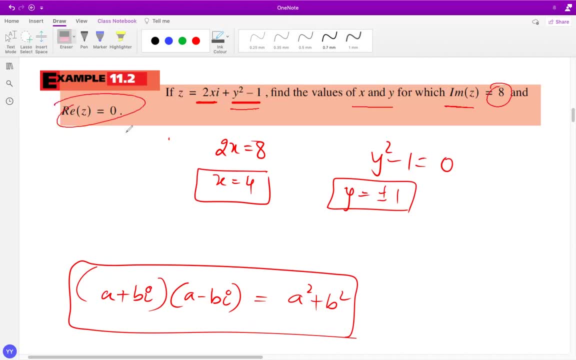 of the complex number is eight and the real part is zero. So when you talk about imaginary part here, so imaginary part is basically two X, because that's a coefficient of the I. we can say So coefficient of I is imaginary part, which is two X is eight. 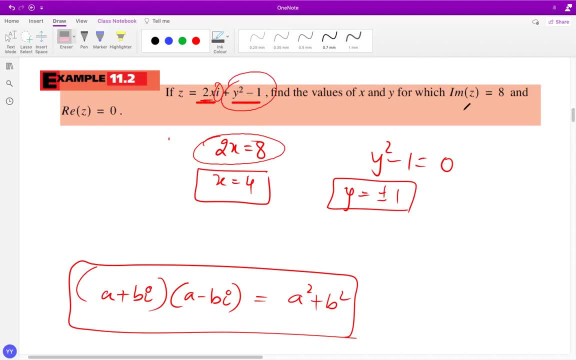 and a real part is Y square minus one, which is zero, because they have given that real part is zero. So if you solve that, you get the complex numbers. That is X equals two, you get four, with Y equals two plus minus one. 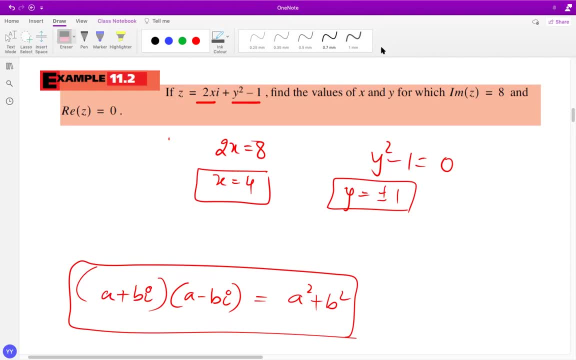 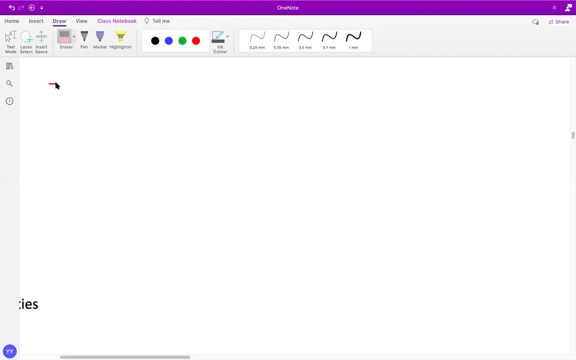 So let's take another example on the property of complex number. So when you add up two complex numbers, the first thing is let's say, if I have a complex number, Z one as two plus four I and Z two is three minus six I. 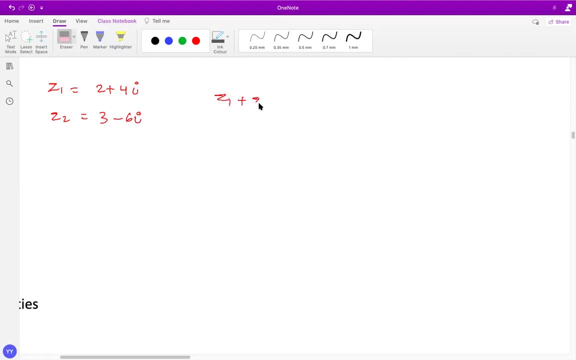 So if I want to add up Z one plus Z two, what's the answer for this? So when you want to add up the complex numbers, you got to add up the real parts. So let's say, if I have two plus four, I plus three minus six, I. 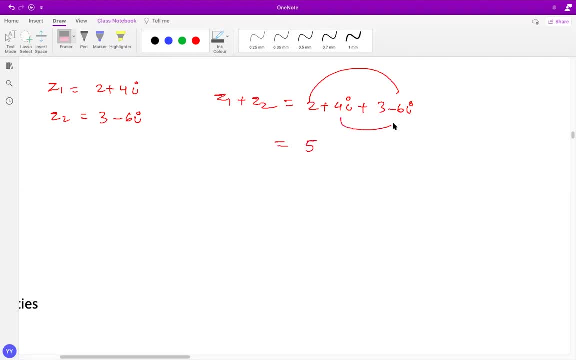 I'm gonna just add up: two plus three, that's your five and four I, minus six I, that's your negative two I. So this is the addition of the complex number. Now, if I show it to you on a diagram now, here it is. let's say, if it is two and four, I. 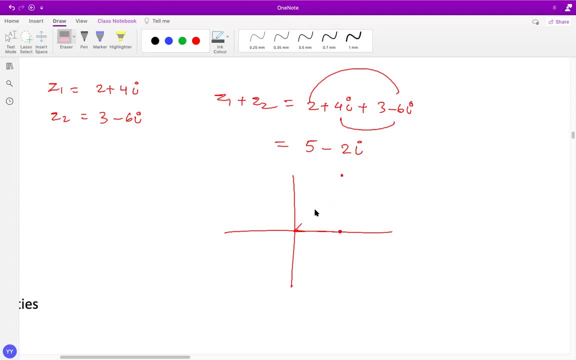 so this is two and this is four. I, this is two, So this is two and this is four. I So this is two and this is four. I. So this is my complex number one, And then I add a complex number three minus six. I. 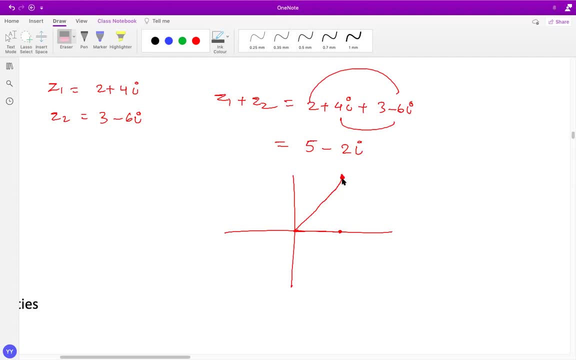 So three minus six I. so this is basically if I say from here: if I add three real that is something and six down, my complex number that I get is something here which is five minus two I. So this is the complex number: Z one plus Z two. 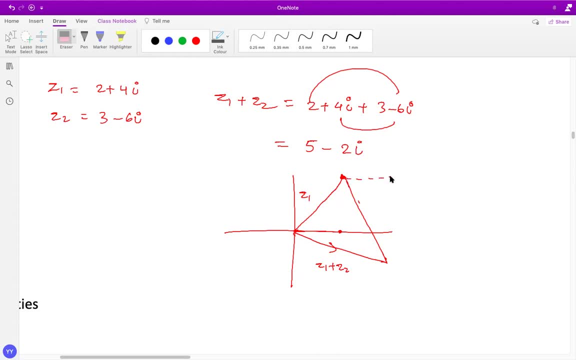 So if this is Z one and if I actually move three to the right and six down here with a second complex number- and here it is actually- I move two to the right and four up. So you go two to the right and four up. 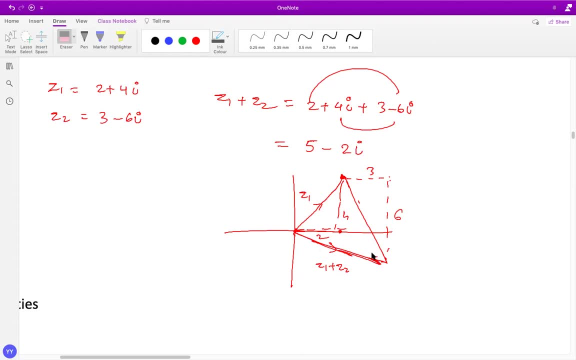 and then you go three to the right and six down. So this is your complex number addition, I would say in that way, So interesting ways, if you can, if you track them as individual, like vectors, like two units to the right and four up. 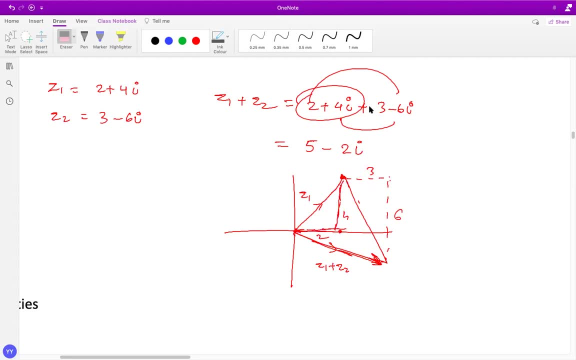 so two to the right and four up, and then three to the right and six down And the resulting complex number you can see is that I went actually over five to the right and this was four, and this was six or two down from the X axis. 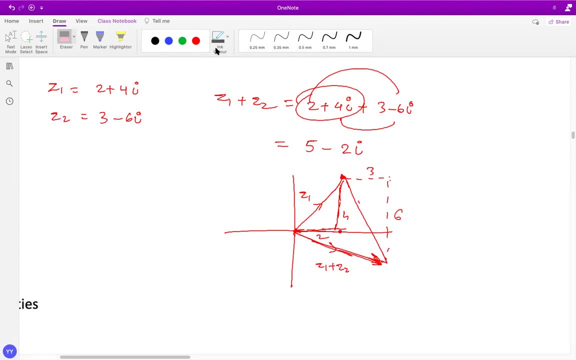 Now next up is: how do you multiply two complex numbers? So when you multiply two complex numbers, it's pretty simple. So Z one times Z two, if you got two plus four, I times three minus six, I when you multiply them. 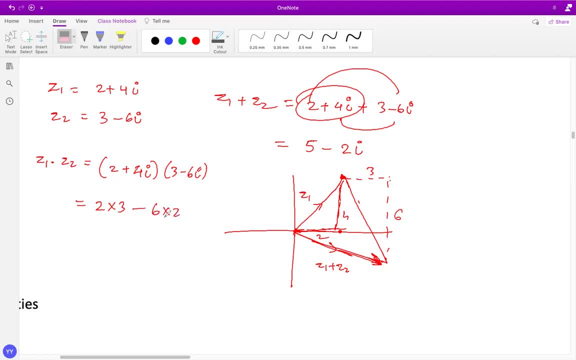 so it is two times three minus six times two, six I times two plus four. I times three minus 24 times I square. So if you simplify this, it is six minus 12 I plus 12 I. If you see here, four threes are 12 I. 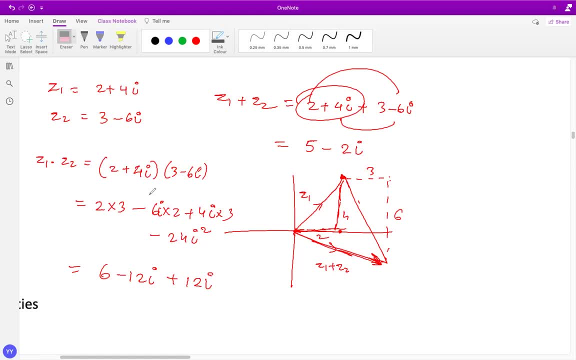 And so, and then here is I square, which is positive 24.. So this is the basic multiplication. So here the answer simplifies to: actually, if you multiply two complex numbers, you get two plus three. I times three minus six. I. 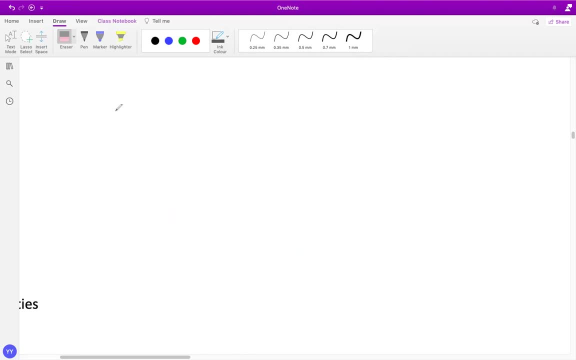 plus four minus six. I times three minus six I. So that's how you multiply and add two complex numbers. Now, if you are subtracting or if you're dividing, it's pretty much the similar logic. So I'm going to take one complex number. 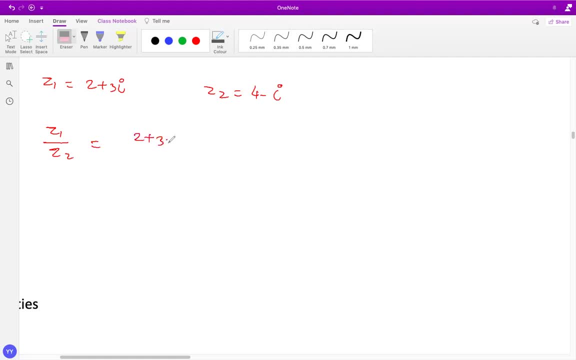 let's say Z one is less than two plus three I and Z two is four minus I. When you divide two complex numbers, Z one over Z two, you get the form A plus B I. So when you have A plus B I format. 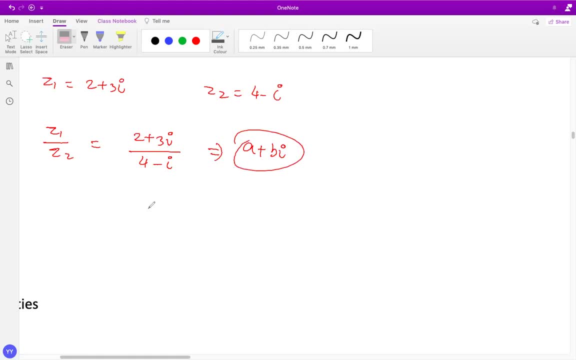 to be written. your answer, in what you're going to do, is: you're going to rationalize this. Okay, you're going to make it. you're going to multiply two plus three I, four minus I times four plus I, over four plus I. 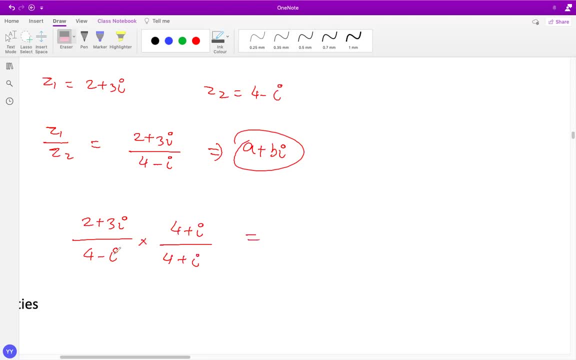 So when you do that, what you get is actually the logic of multiplication here is that this is A minus B and this is A plus B, And this is referred as a complex conjugate. So when you multiply, this is A minus B and this is A plus B. 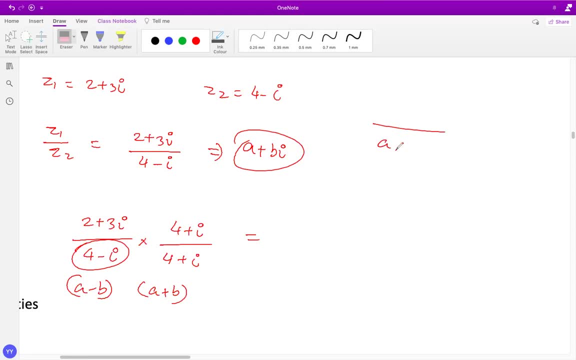 And this is referred as a complex conjugate. So when you multiply, actually if it is in denominator, if you got A plus B I, you got to just change the sign of the imaginary part and multiply with A minus B I and divide by A minus B I. 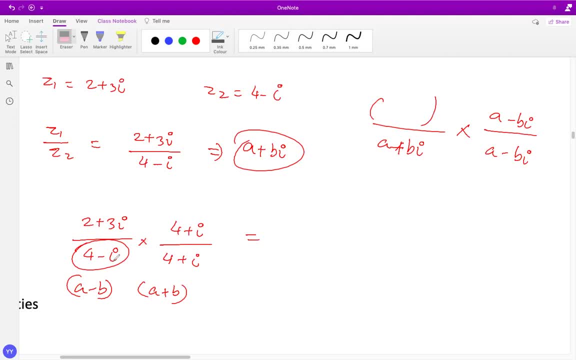 Whatever is in numerator, it doesn't matter. So for us it is really important. And by doing so, if you look at, this is A square minus B square in denominator. So what we get is two plus three I in numerator and four plus I in numerator here. 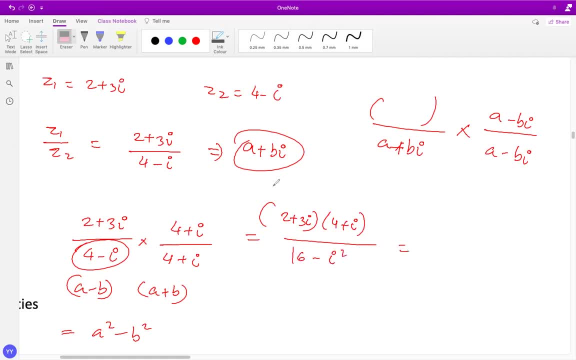 And then you got 16 minus I square. So what we get is actually eight plus two I and plus 12 I and plus three I square, or 16 minus one, which is 17, because I square is negative one. So 16 plus one actually is 17.. 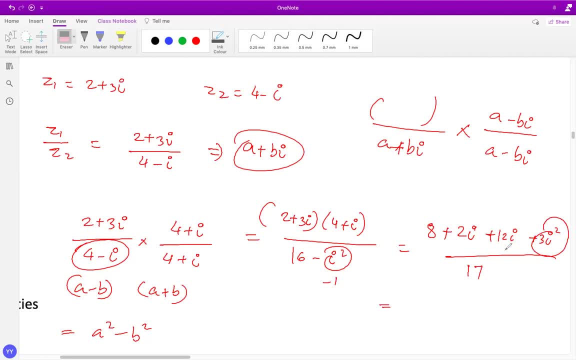 So here what we get is: in numerator we get eight minus three, which is five, and 12 plus two is 14.. So what we get is: this is a rational denominator here. So this is how you do the conversion from this form to this form. 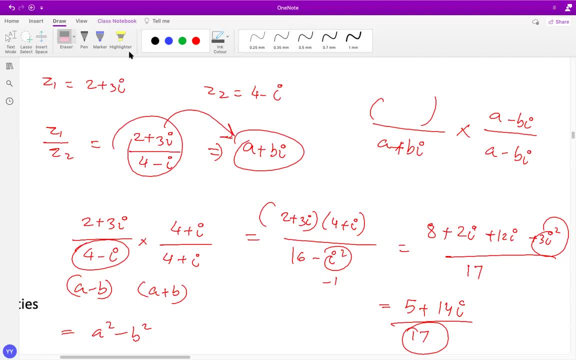 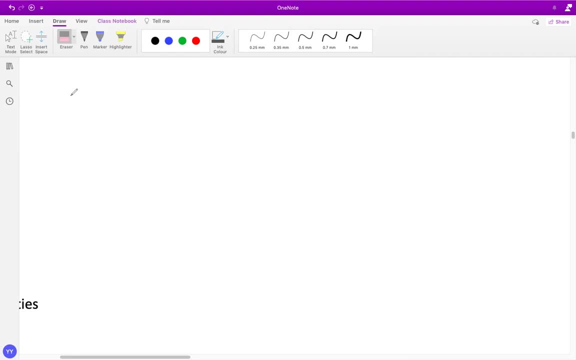 It's also referred as division of complex numbers. So I hope this basic properties are clear to you. Now I'm just gonna take a little bit about something called as conjugate of a complex number. Now, if you talk about conjugate of complex numbers, 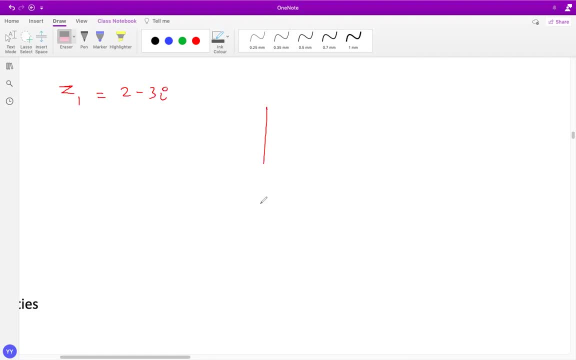 so let's say, if I have Z one as two minus three, I So, if I show it on the Argon diagram, Z one is two minus three minus three. I So two units to the right and three units down. So that's where is my complex number. Z one is: 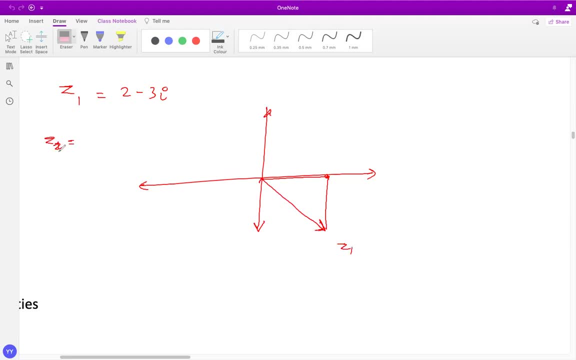 I'm gonna look at Z two and which is actually Z one star. we say sometimes Z one star or sometimes it's Z one bar. That means the conjugate, And conjugate is written as by just making the imaginary part positive. 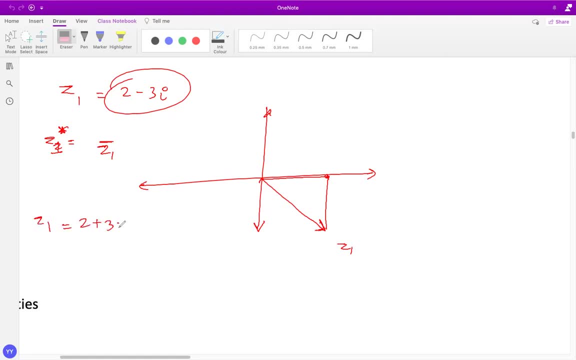 So like let's say: okay, the conjugate of Z one is gonna be two plus three I, That's conjugate here, And if I have conjugate of, let's say, a complex number, So okay, I'm just taking another example here. 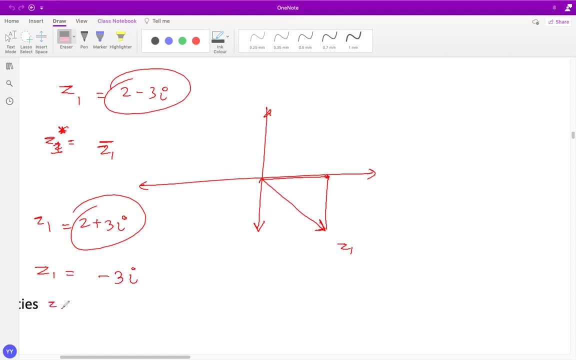 Like, okay, complex number is negative three, I. My conjugate will be Z. one star is gonna be three, I. So you just can change the imaginary part positive or negative based on the sign. So actually it is just out here. So this is the conjugate of the complex number. 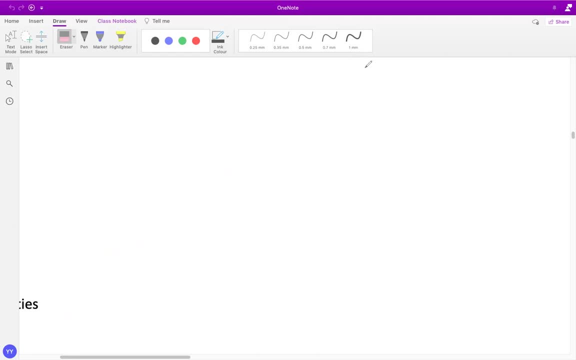 And next property that I wanna cover up about complex number is something called as the modulus and argument. Now, if I refer as a complex number Z, A plus B, I, Now my modulus and argument is actually, if you look at the A part: 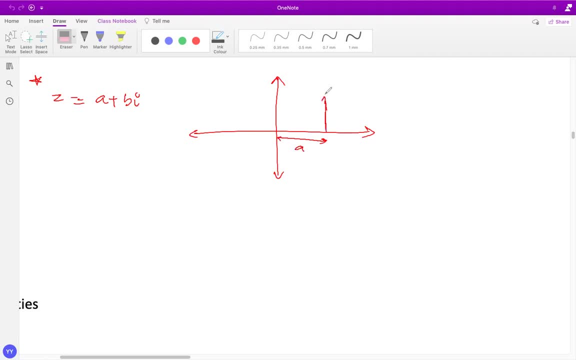 the real A part is A and imaginary part is B. So here is imaginary part And this is my complex number. assume Now the modulus of the complex number is defined as the square root of A square plus B square, according to Pythagoras theorem. 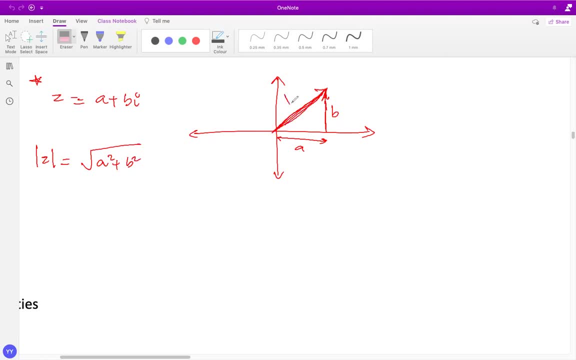 That's actually can think about in this way. it's the length of the complex number. So this is the. it's referred as modulus, like two bars is representing the modulus, or sometimes it is referred as R. So when you talk about a complex number, 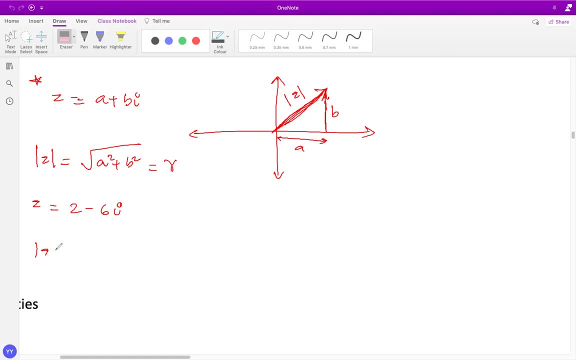 as Z is two minus six, I, the modulus of this complex number, is two square plus minus six square and the root of the whole thing. So that's the root of four plus 36, which is square root of 40. So any complex number if you got like. 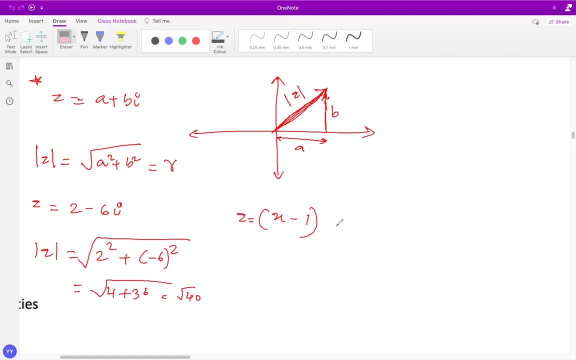 suppose if I got X minus one, Z is X minus one plus three. I, the modulus of this is X minus one, the whole square plus three, square the root of this. So this is the modulus of this complex number. So this as far as the basic properties are concerned. 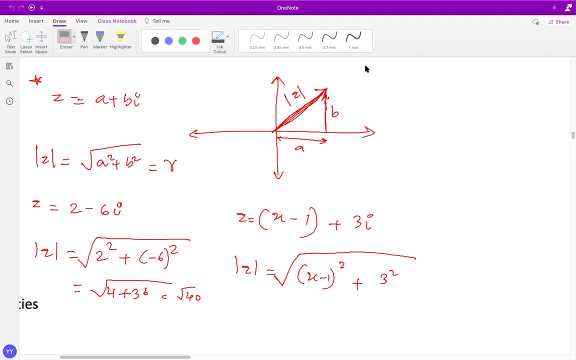 this is the modulus And I'm gonna take the next part is something on argument. Now to find the argument of a complex number. what we got to do is we got to be very careful about something. What is argument First? So argument when you talk about argument of complex number. 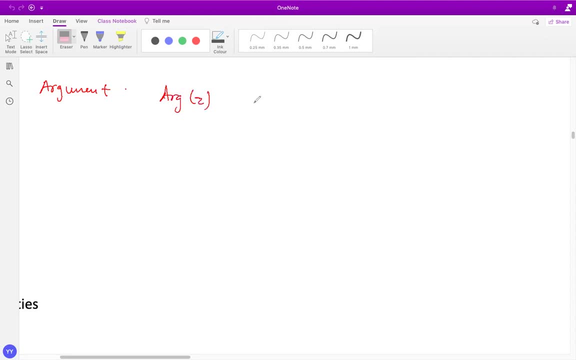 or let's say arg Z- sometimes we write down- or small arg Z, So this is something which you got to understand very briefly. Now, when you talk about the complex number, I have my own way of finding the argument of complex number. 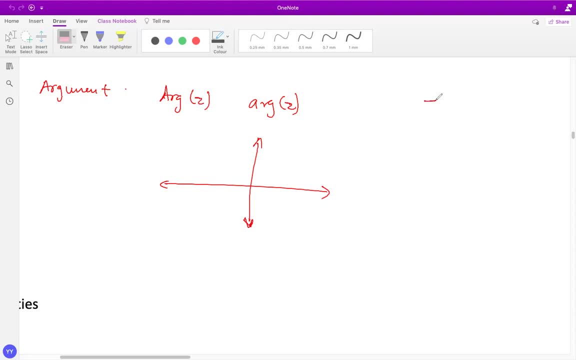 So first thing is that when you write in the argument you got to be very careful that an argument of a complex number must be between negative pi to pi, So negative pi to pi and the pi is inclusive and negative pi is not included. 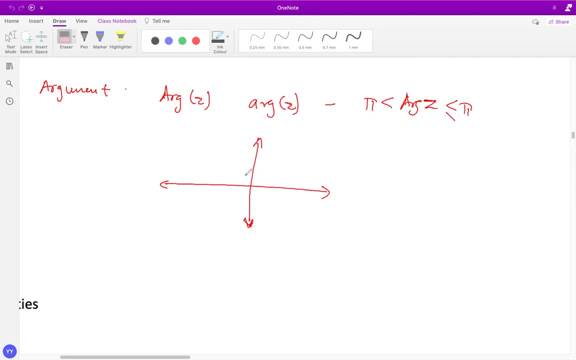 So here, what is argument that I'm talking about? So first assume that, let's say, complex number is in the first quadrant. Now, when you talk about the argument here, I just think about this angle that is made with the positive direction of X axis. 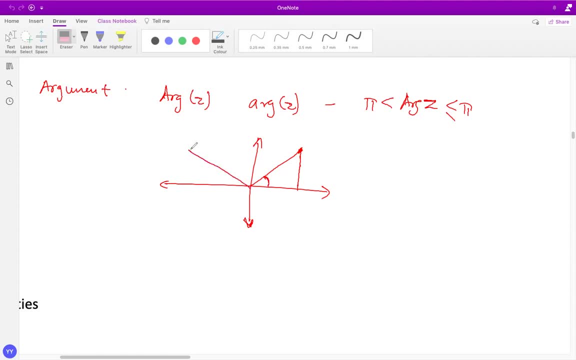 If my complex number is here, my argument is actually this: If my complex number is here, my argument is this: or I can take this, but there is some clarity about this. Okay, There is something that I want to clarify in later part of the video. 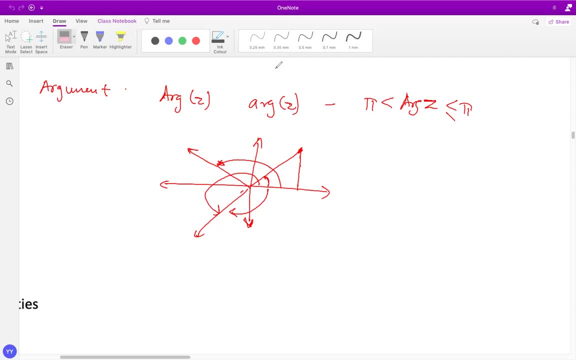 So how do I define argument? Now, actually, if you look at the argument, is the angle made with the positive direction of X axis by the complex number, if my complex number is actually, let's say, in any particular quadrant. what I need to do is I just need to find out. 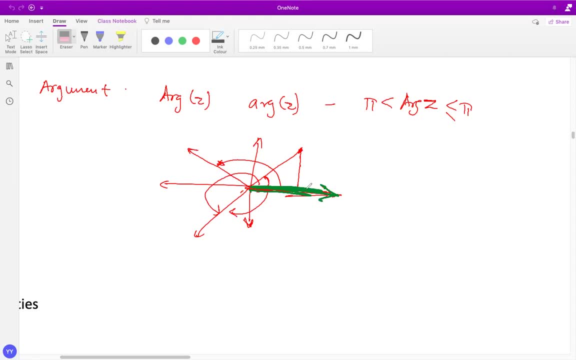 what is the angle made with the positive direction of X axis? So let's take an example: how to find out the argument of a complex number. So before I generalize for Z equals to X plus IY, I want to take an example. 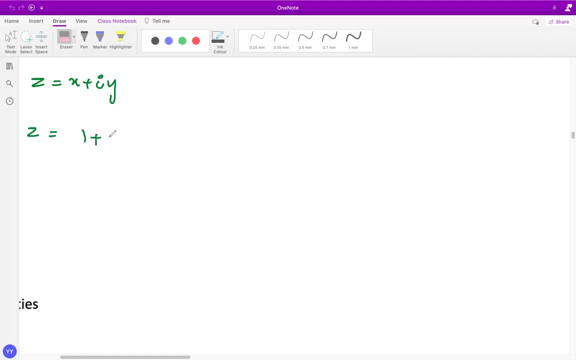 like let's say one plus, let's say I, Now one plus I is I'm gonna be in first quadrant here. Now that complex number is actually gonna be here, one unit along X axis, I mean the real axis, and one along imaginary. 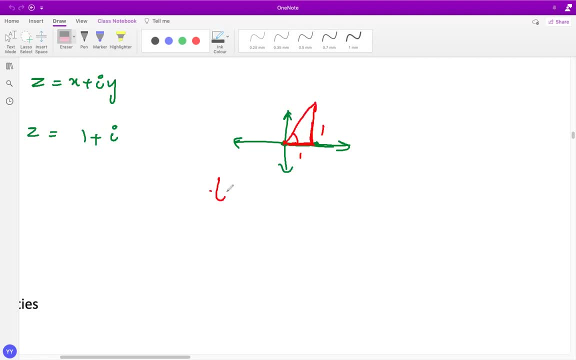 So that's here it is. The angle is tan theta. If I take this angle as theta, the tan theta is one over one which is opposite or adjacent. So theta is pi by four. So here is my argument, Now what we got to understand. 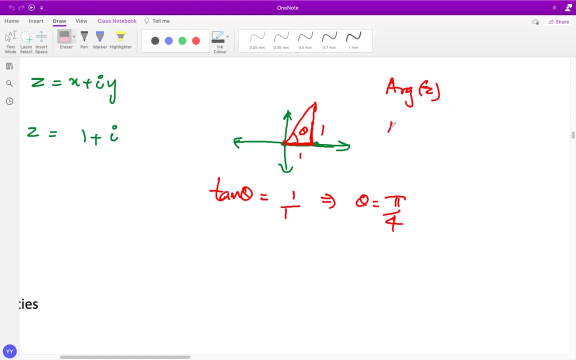 is the difference between capital RZ and small RZ. So when you're writing the argument of a complex number, one of the argument is referred as a principal argument, So that is shown by capital ARZ. Now what is the principal argument? 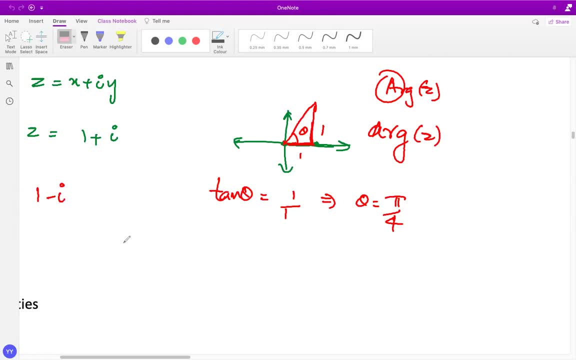 Now, if I have a complex number in one minus I, let's say, when I'm finding out one minus I. Now, when I look at the angle here, now if I represent it on the argon diagram, my complex number is actually gonna be somewhere here. 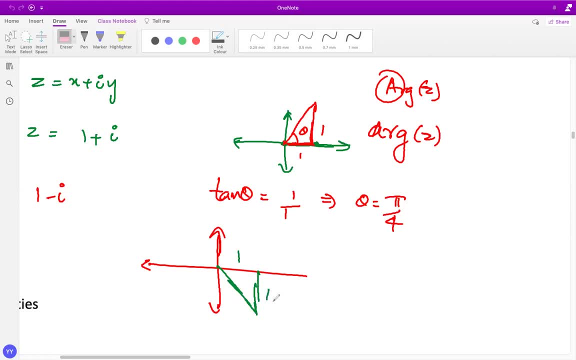 So that's your one and one again. I mean this is negative one, but it's length I'm just taking, So here actually I can take argument at this angle. So this angle is actually, if I write down this, tan theta is one over one. 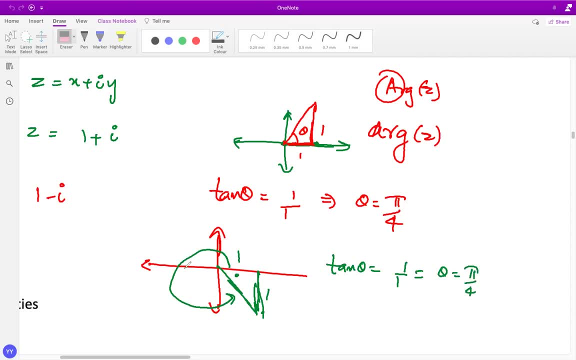 So theta is pi by four. So this angle is actually. this angle is pi by four. Now, when you find out this angle, is pi by four actually from here, if I find out this angle, it is gonna be two pi minus pi by four. 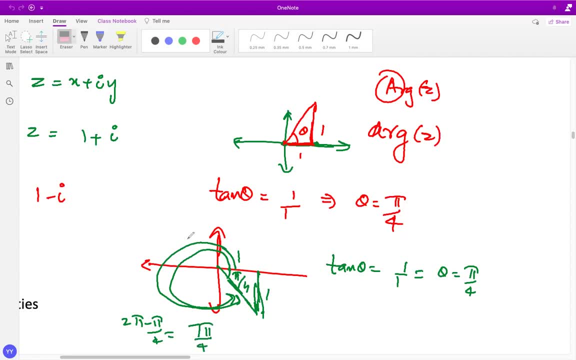 which is gonna be seven pi by four. So I can say: okay argument of this complex number is actually seven pi by four. But as per the condition of the principal argument, this must be between minus pi, two pi, And this pi is included. 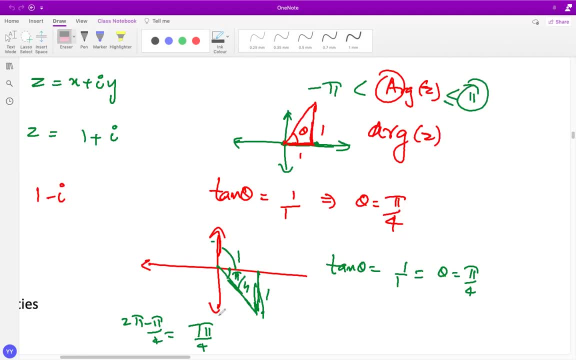 And minus pi is not included Now. so if it is not between negative 180 to 180, or negative pi to pi, it is not referred as a principal argument. So what we got to be careful here is so I don't take principal argument as seven pi by four. 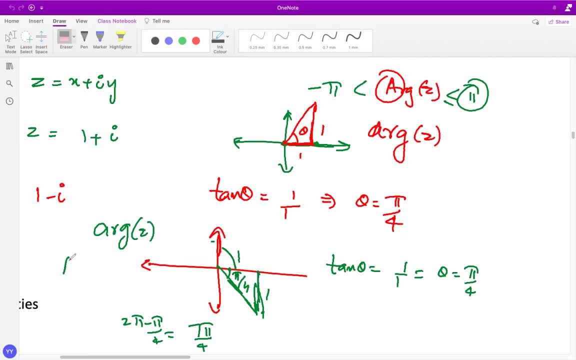 Okay, that is gonna be small ARG, okay, But when you write in capital, ARG, okay, of a complex number, what are you gonna take? is you're gonna take this complex number, That is, this part which is negative pi by four. 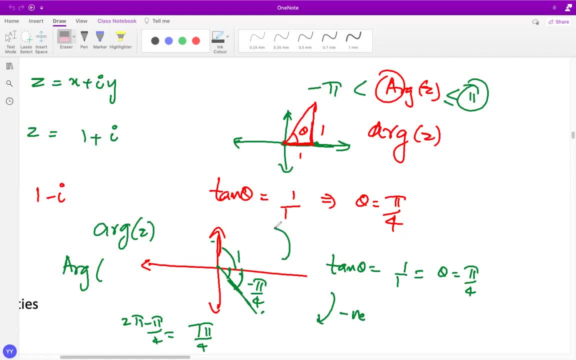 So when you go clockwise, you take the angle negative. When you go anti-clockwise, you take angle positive. So that's why this angle is the argument, principal argument of one minus I, which is so if I write an ARG of one minus I. 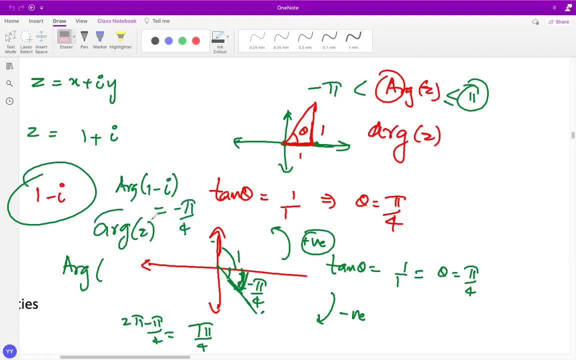 it is negative pi by four. Of course I can write down like this: which is seven pi by four as well, But that won't be capital ARG, that'll be small ARG. So now let's take some more example about the argument.